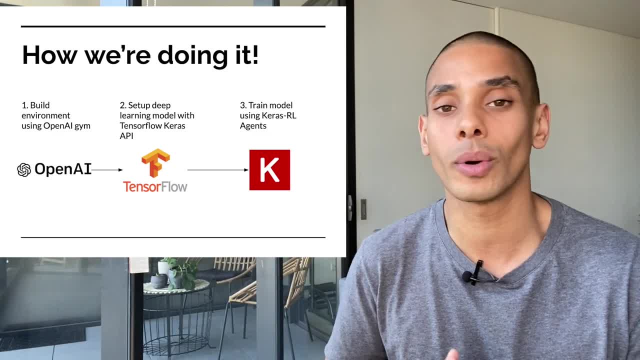 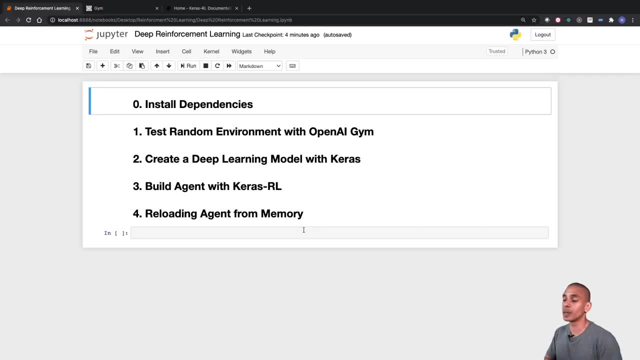 take that same model, save it down into memory and reload it for when we want to deploy it into production. Ready to get to it, Let's do it. So there's a couple of key things that we need to do in order to build our deep reinforcement learning model. So, specifically, we need to first up, install. 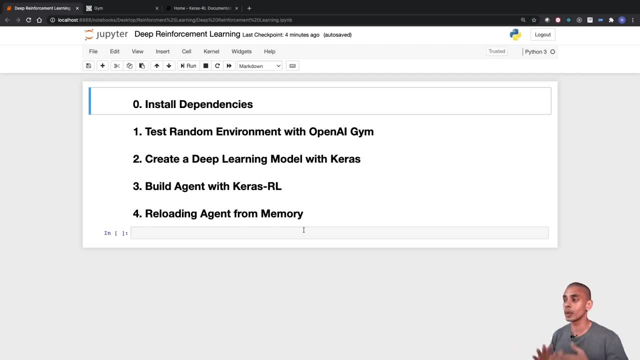 our dependencies, then what we're going to do is build an environment with OpenAI Gym with just a couple lines of code. So this is going to allow us to see the environment that we're actually using reinforcement learning. in later on, Then we're going to build a deep learning model with Keras. 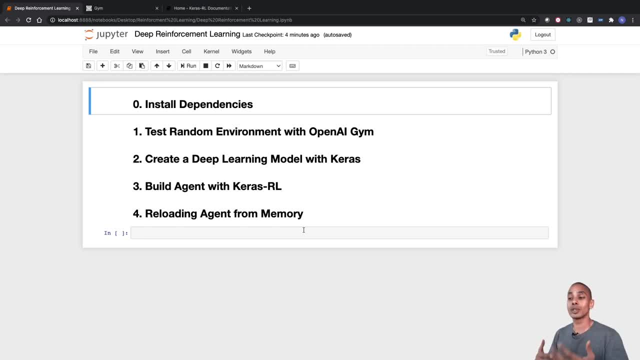 we're going to be using the sequential API there, and then what we're going to do is train that Keras model using Keras reinforcement learning and, last but not least, we're going to delete it all and reload that agent from memory. So this is going to allow you to deploy it into production. 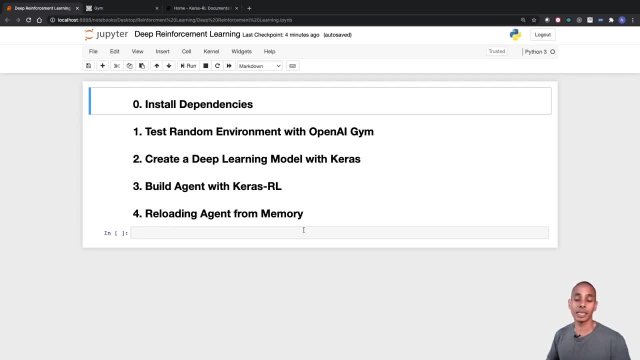 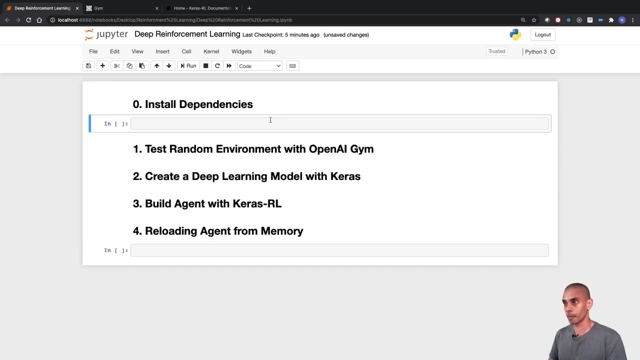 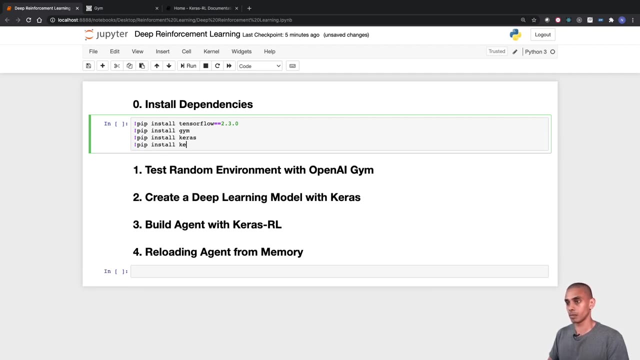 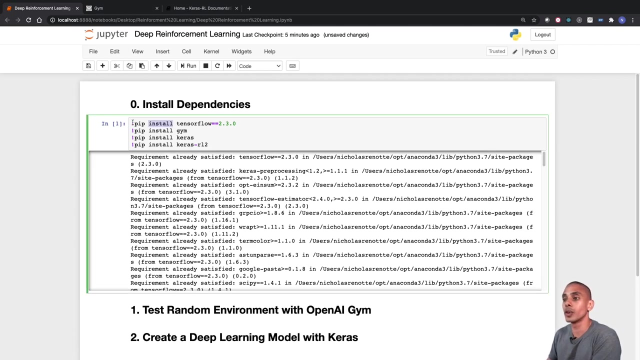 if you want to later on. So first up, let's install our dependencies. So what we're going to need here is TensorFlow, Keras, Keras RL, as well as OpenAI Gym. So what we've done is we've installed our four key dependencies. So we've used pip install and 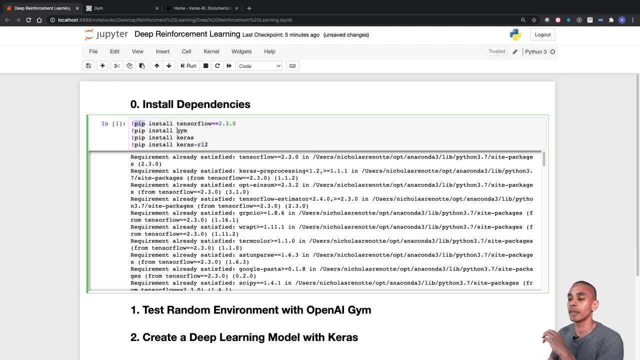 specifically, we've installed TensorFlow 2.3.0.. We installed OpenAI Gym, so that's just Gym. We've installed Keras and we've also installed Keras RL2.. So those are all our dependencies now done and installed. Now what we can actually go and do is set up a random environment with. 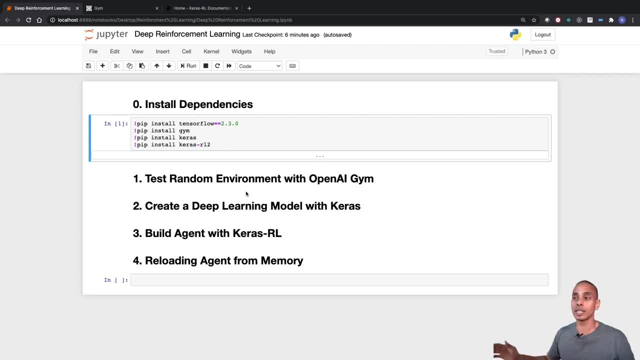 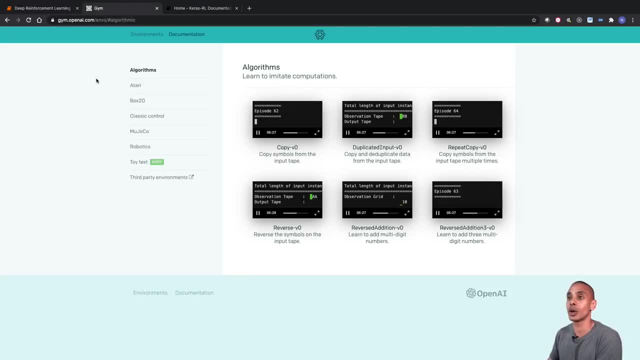 OpenAI Gym. Now OpenAI Gym comes with a bunch of properties that we can install. So we can install pre-built environments that you can use to test out reinforcement learning on. So if we actually head on over to gymopenaicom you can see there's a bunch of random environments. So here we've got. 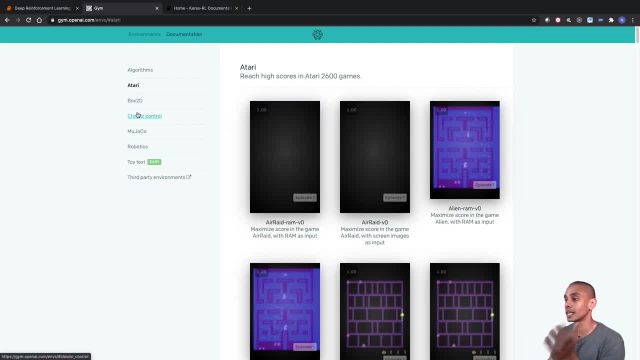 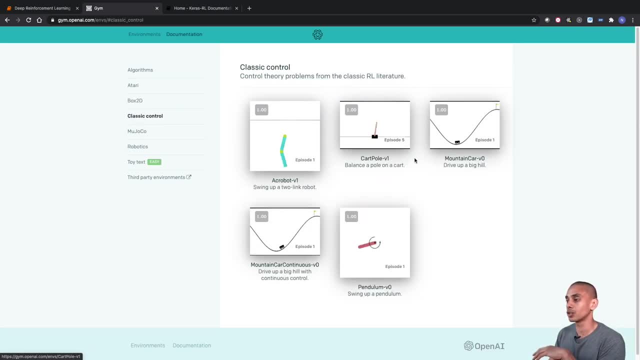 some algorithms. we've got Atari games, So if you wanted to build Atari or video game style reinforcement learning engines, you could. We're going to be working on these classic control ones and specifically, we're going to be using CartPole, And so the whole idea behind CartPole is that you 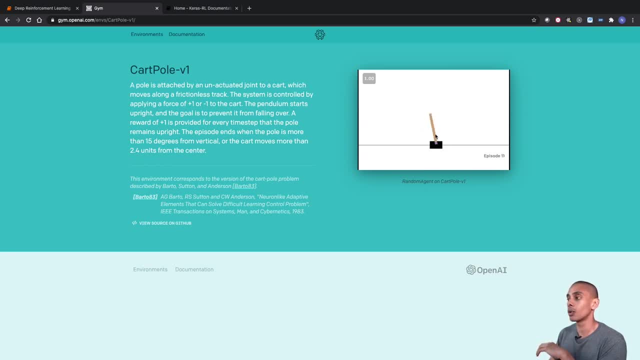 want to basically move this cart down the bottom here in order to balance the pole up there. So the whole idea is that for each step you take, you get a point, with a maximum of 200 points. So ideally, what we're going to see when we start off is, with our random steps, we're not going to get anywhere near 200. 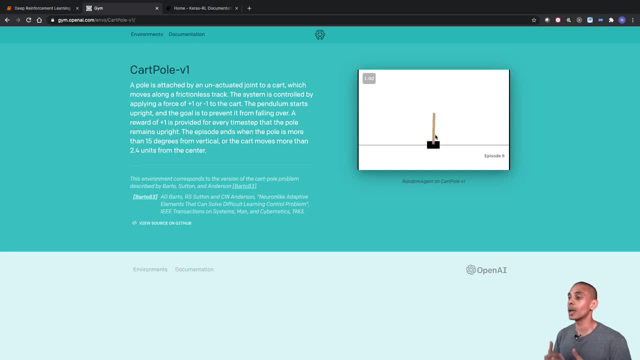 but once we use deep learning and reinforcement learning, we ideally should get a much closer to actually hitting our final result. Now we've got two movements. we can either go left or right. So what we're going to see is when we create our environment. we're going to have two. 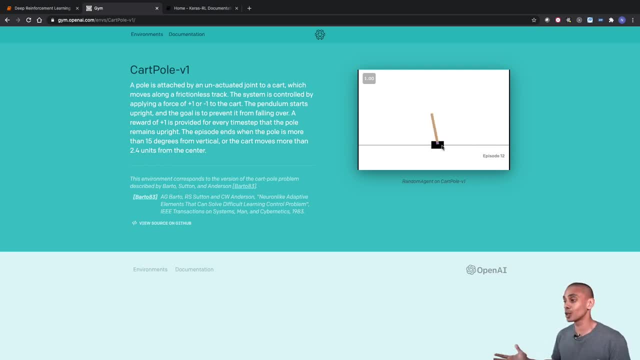 actions available, either left or right. If you work in different reinforcement learning environments, you might have a different number of actions that you can take. So, for example, you might go up or down, left or right if you're working with other things. So now what we're. 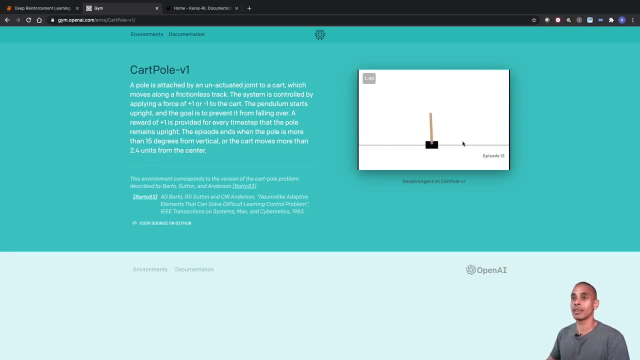 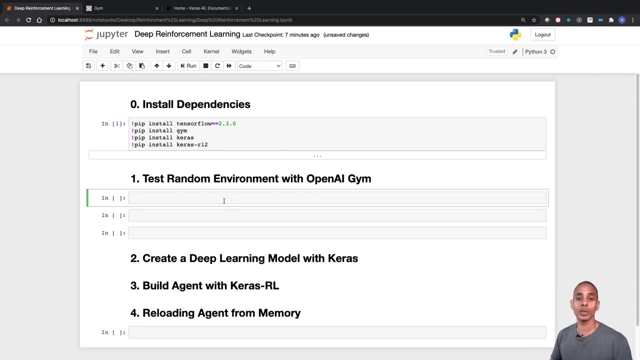 going to do is set up this environment so you can work with it within Python. So if we go back to our Jupyter notebook, let's start setting that up. So the first thing that we need to do is import our dependencies. So in order to do that, we're going to import OpenAI Gym and we're also going 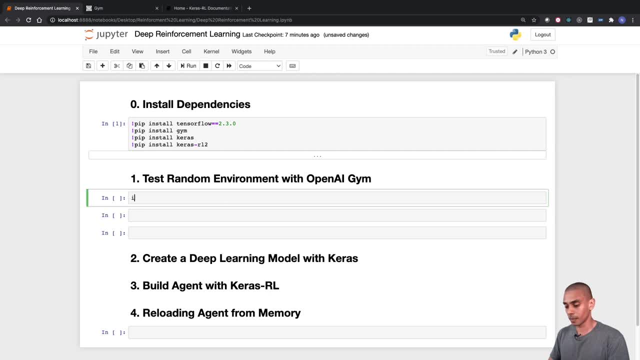 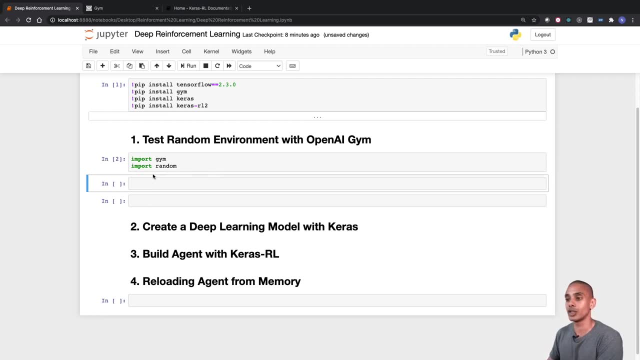 to import the random library so we can take a bunch of random steps. So those are our two key dependencies imported. So, and this is specifically for our OpenAI Gym, So we've imported Gym and we've also imported random. Now what we can go and do is actually 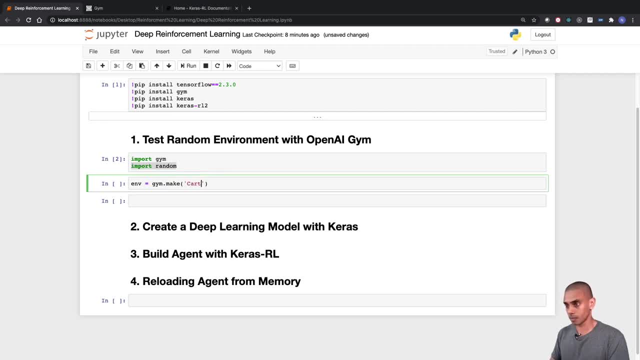 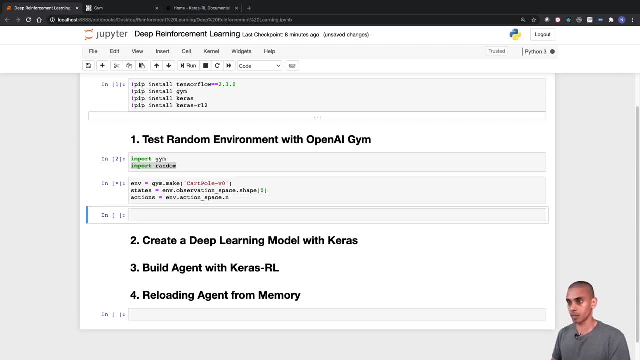 set up that environment. So that's our environment set up. So what we went and did there is we used the OpenAI Gym library and, specifically, we used the make method to build our cartpole environment. So remember, that was the cartpole environment, that. 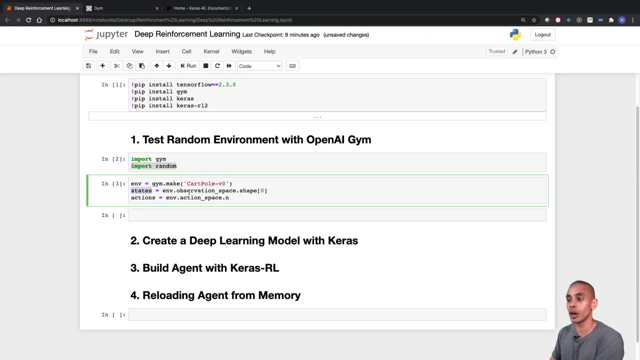 we saw here. We then extracted the states that we've got. So this is available through ENV, which is our environment that we just set up Observation space dot shape. So we're taking a look at all the different states that we've got available within our environment and we've also extracted the 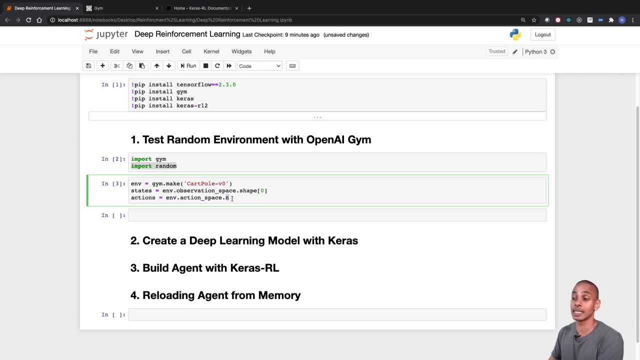 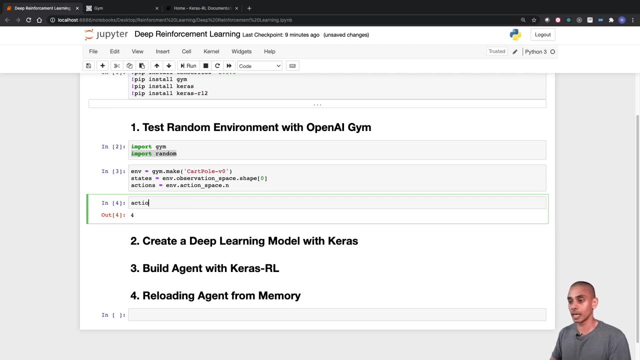 action. So if you take a look, we're getting that from our action space and we can see that we're going to have a specific number of actions. So if we take a look at our states, we've basically got two actions available. And if we take a look at our actions, we've got two actions. So basically, 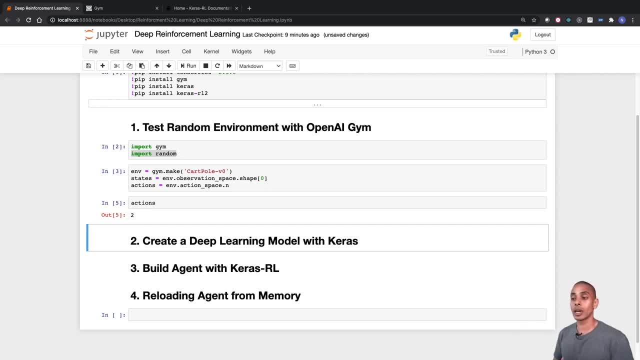 those are left or right, moving our cartpole left or right. Now what we can actually go and do is actually visualize what it looks like when we're taking random steps within our cartpole environment. So ideally, what we'll see is that our cartpole is just sort of moving randomly because we're taking 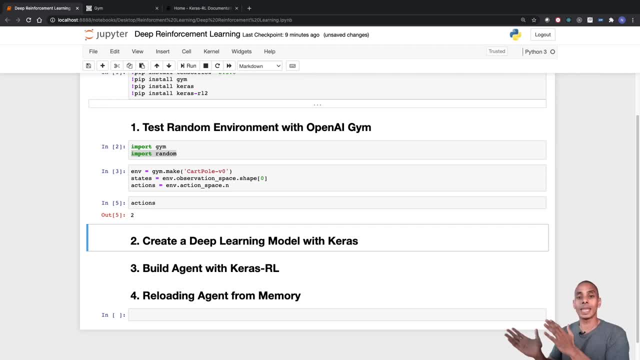 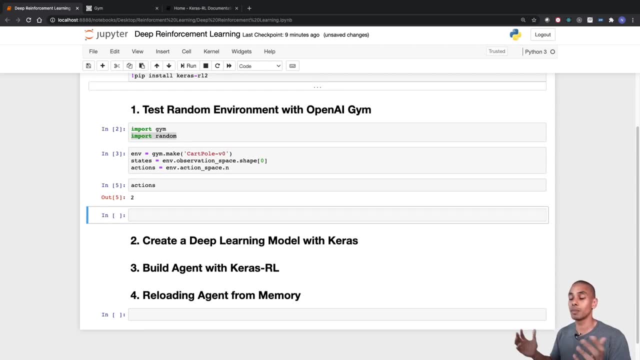 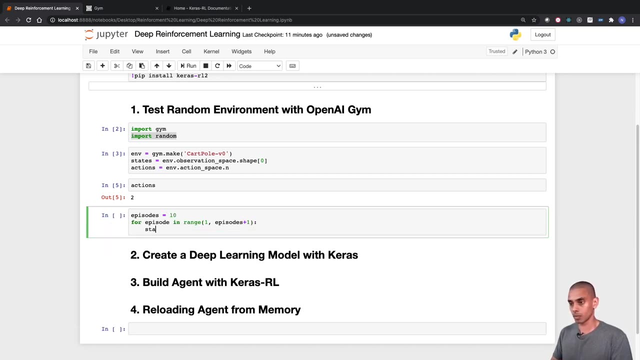 random steps in order to get a specific score. So remember, with each step that we take where our cartpole hasn't fully fallen over, we're going to get one point with a maximum of 200 points. So let's build our random environment. 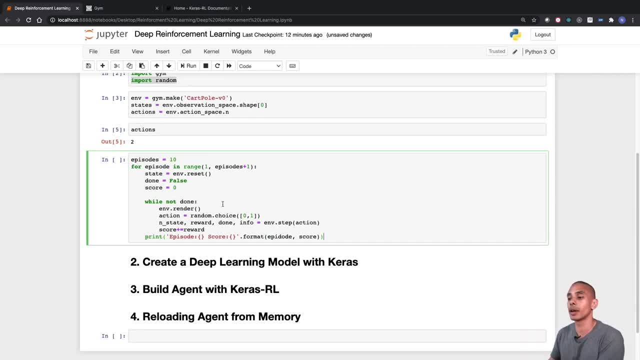 Alright, so we've written a bit of code there. Now what we're actually going to do is start by breaking this down from here. So the first thing that we're going to do is render our environment. So this is going to allow us to see our cart in. 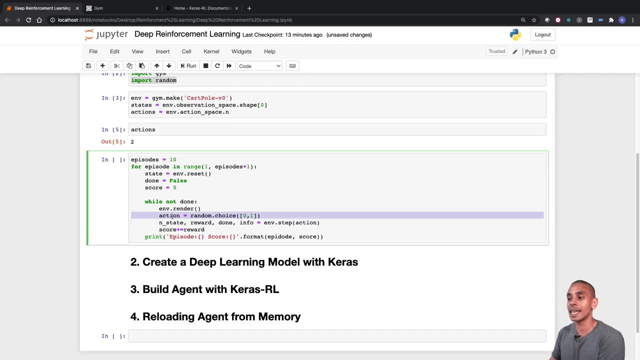 action when it's moving left and right, Then what we're doing is we're taking a random step, So we're either going left or right, So zero or one basically represents one of those steps. So we're just taking a random choice to see how that impacts our environment. Then what we're doing 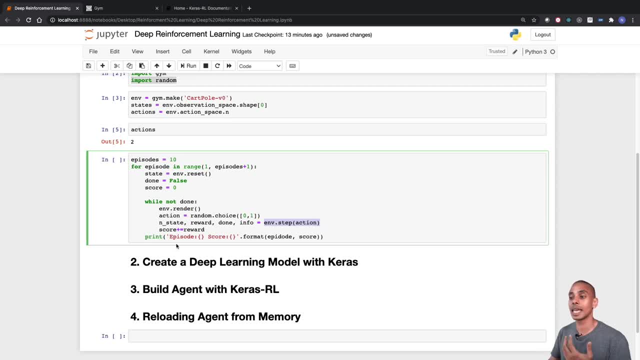 is we're actually applying that action to our environment and we're getting a bunch of stuff as a result of that. So we're getting our state, we're getting our reward, we're getting whether or not we've completed the game. So, whether or not we've failed or whether or not we've passed, 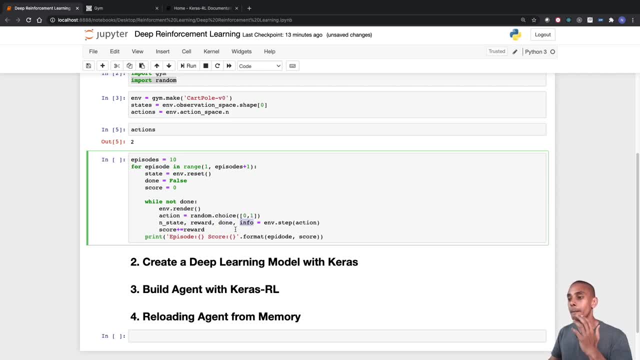 and we're also getting a bunch of information. Then, based on our step, we're going to get a reward. So remember, if we take a step in the correct direction and we haven't failed, we get one point. This basically allows us to accumulate our entire reward. Now, if we fail or if we get to, 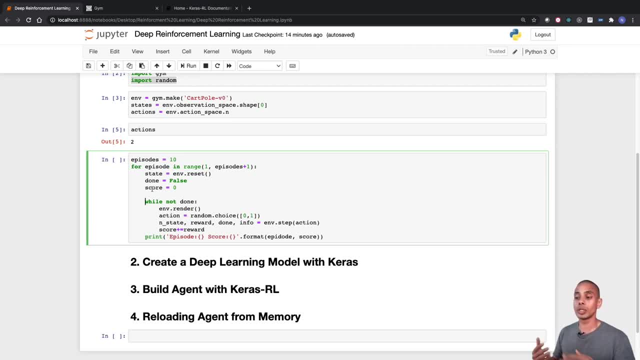 the end of the game, then done is going to be set to true. So what we're doing is we're continuously taking steps and we're getting a reward. So what we're doing is we're continuously taking steps until we're complete. So we reset the entire environment up here and then we're also printing. 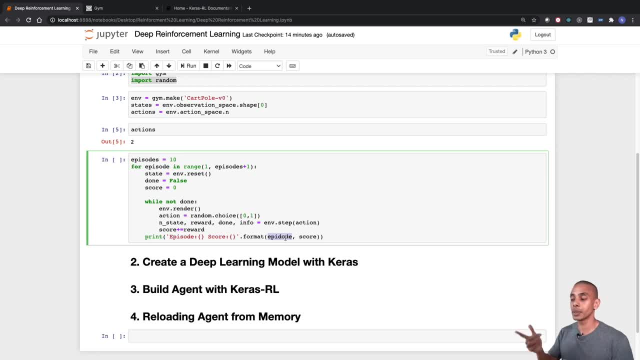 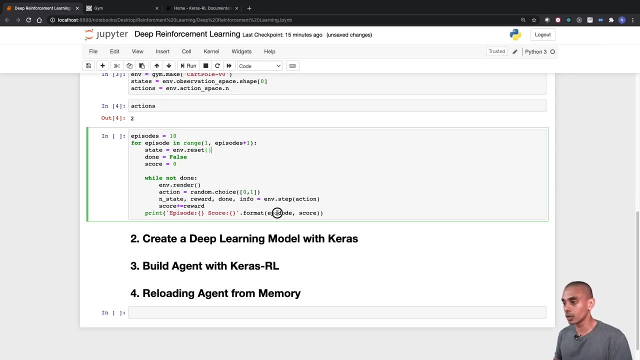 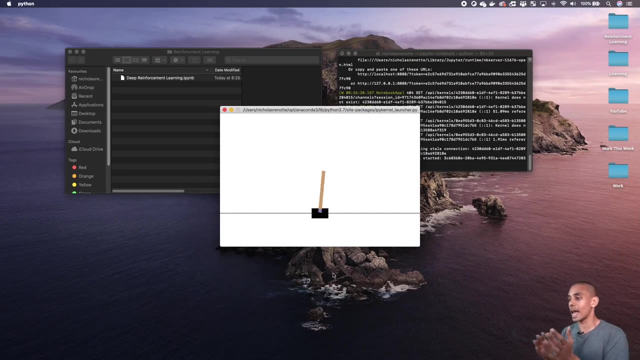 out our final reward. So ideally, what we'll get is the episode number as well as our score. So let's go on ahead and run that and see our episodes live and in action. Actually, it looks like we've got a bug there. episode All right, so you can see our cart's moving and it's moving. 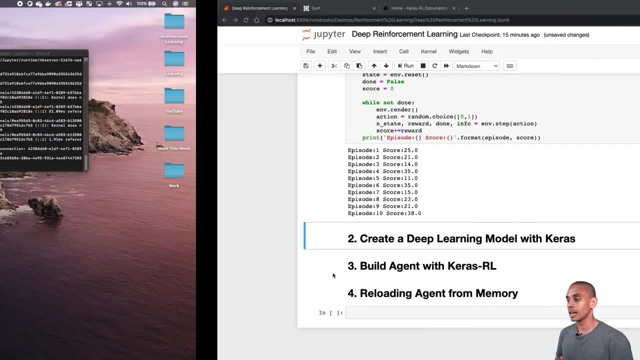 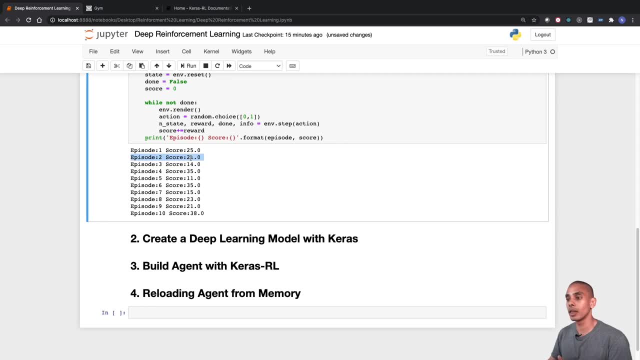 randomly, and you can see that our poll is sort of flailing about Now. what we're actually logging out is the score, So it looks like we're surpassing a specific threshold and we're failing, So we're only getting up to a maximum of about 38.. So that's our maximum score. Now, ideally what we want to. 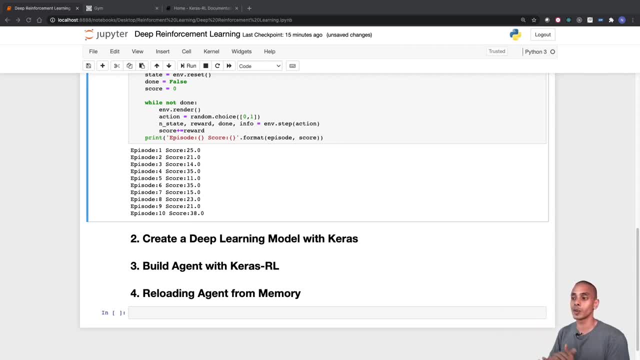 be able to get is all the way up to 200, and this is where reinforcement learning comes in. So, basically, our deep learning model is going to learn the best action to take in that specific environment in order to maximize our score. Now, this all starts with a deep learning model, So 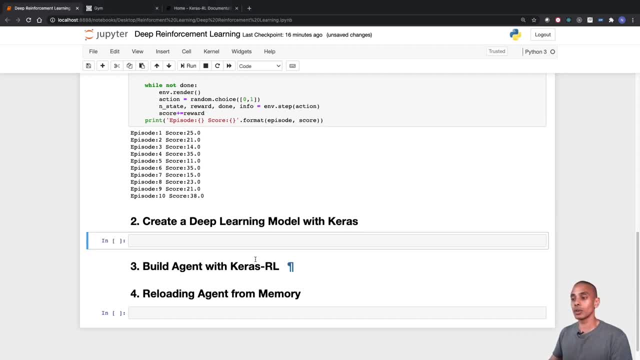 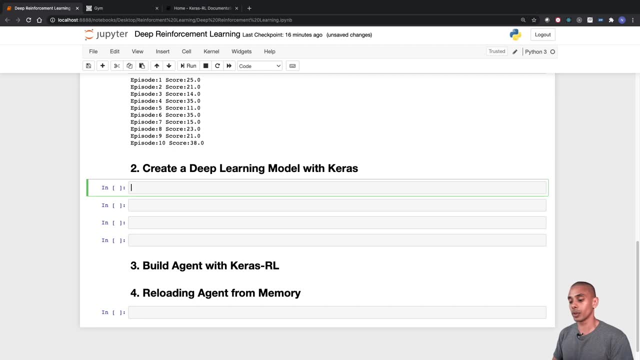 let's go on ahead and start creating our deep learning model Now. in order to do that, we first up need to import some dependencies. So let's go ahead and start creating our deep learning model. So we've imported our dependencies, So let's go on ahead and import those. 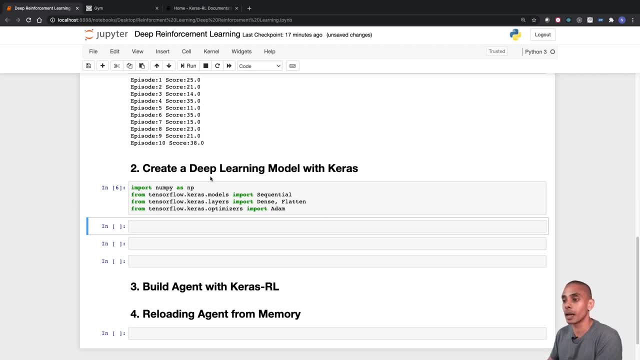 So we've imported our dependencies. So we've specifically first up imported NumPy, So this is going to last work with NumPy arrays. Then we've imported the sequential API. So this is going to last build a sequential model. So this is going to last build a sequential model. 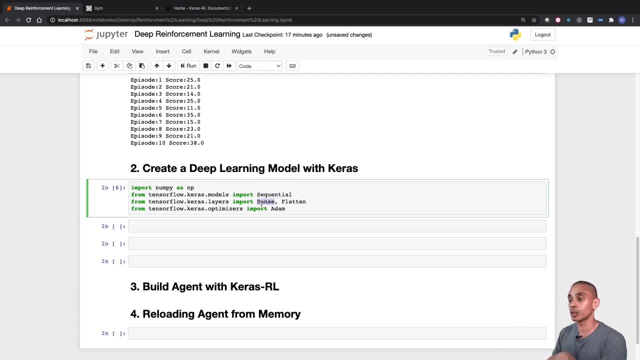 model with Keras. then we've also imported two different types of layers, so specifically, we've imported our dense node as well as our flatten node. and, last but not least, we've imported the atom optimizer. so that's going to be the optimizer that we use to train our deep learning model. now. 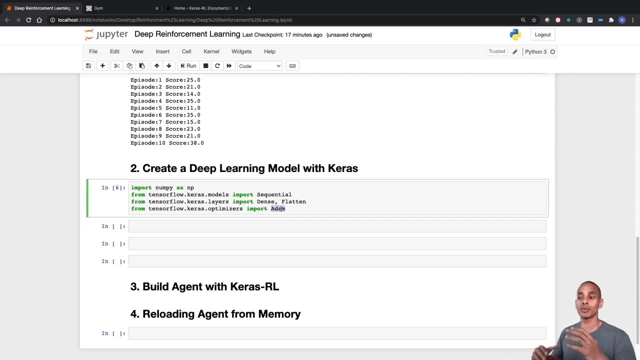 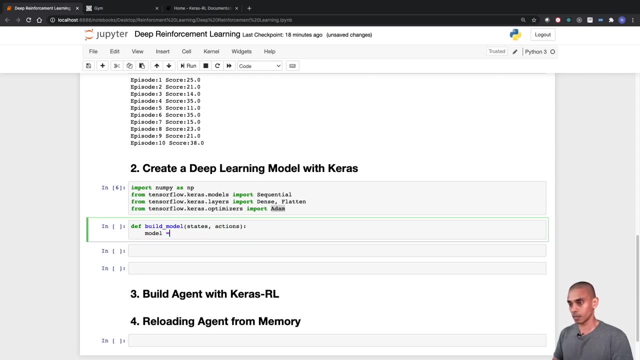 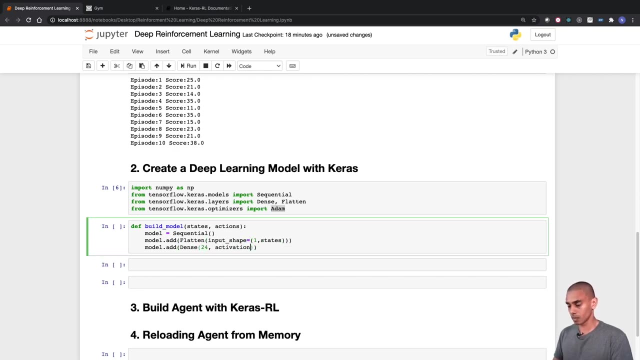 what we can go and do is actually go and build that model. so we're going to build this wrapped inside of a function so we can reproduce this model whenever we need to. so that's our build model function defined. so what we've basically gone and done is created a 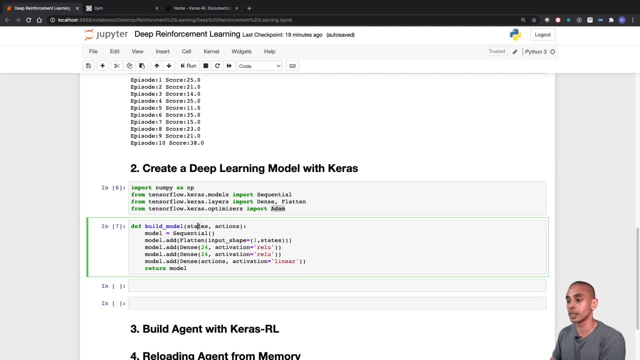 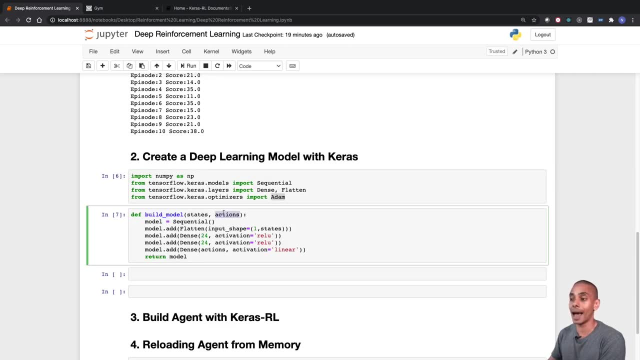 new function called build model, and to that we're going to pass two arguments. so specifically, our states. so these were the states that we were going to use to train our deep learning model. we extracted from our environment up here and we're also going to pass through our actions. 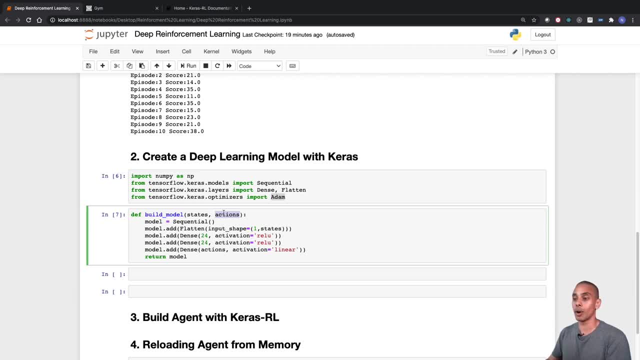 so these are going to be the two different actions that we've got in our carpool environment in order to build our deep learning model. we're first instantiating our sequential model, then we're passing through the flatten node and specifically to that we're going to be passing. 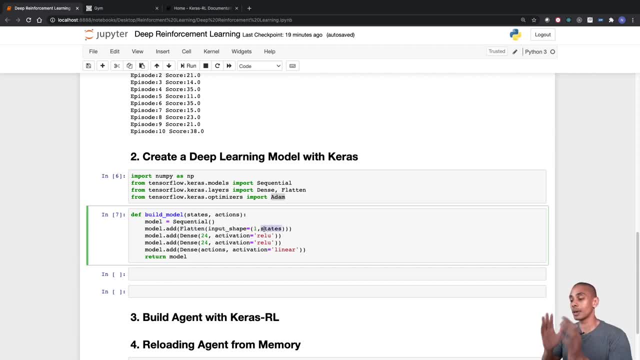 through a flat node which contains our different states, so remember our four different states that we had. then we're adding two dense nodes to start building out our deep learning model with a relu activation function. and, last but not least, we're going to pass through a flatten node. 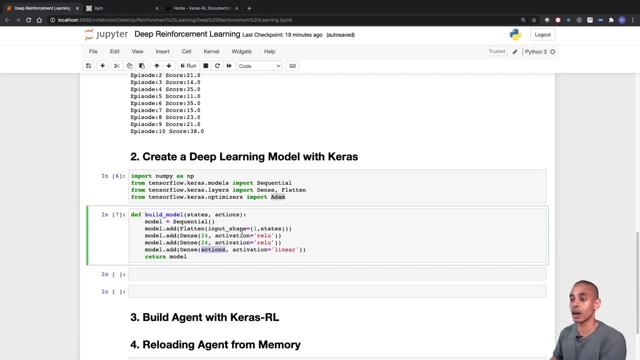 which contains our last dense node, has our actions. so this is basically going to mean that we pass through our states at the top and we pass through our actions down the bottom. so, ideally, what we should be able to do is train our model based on the states coming through to. 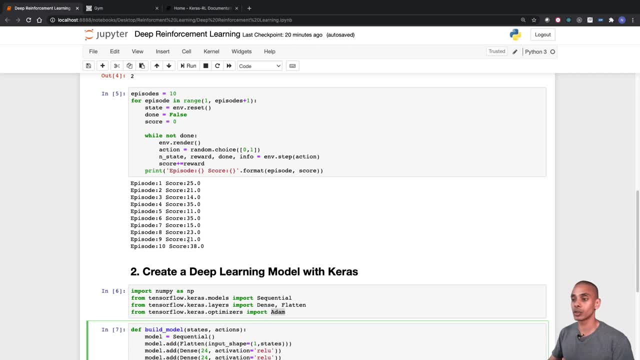 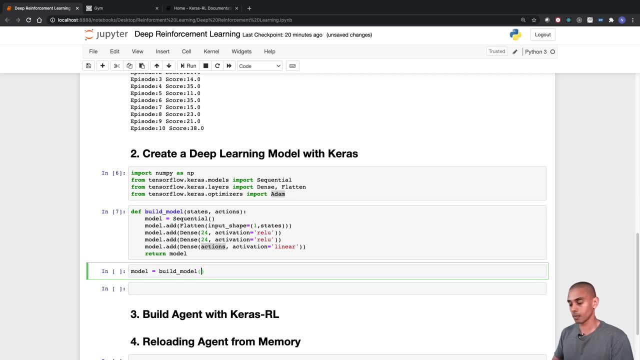 determine the best actions to maximize our reward or our score that we can see here. so let's go on ahead and create an instance of that model just by using that build model function. and we can also visualize what the model looks like using the modelsummary function. 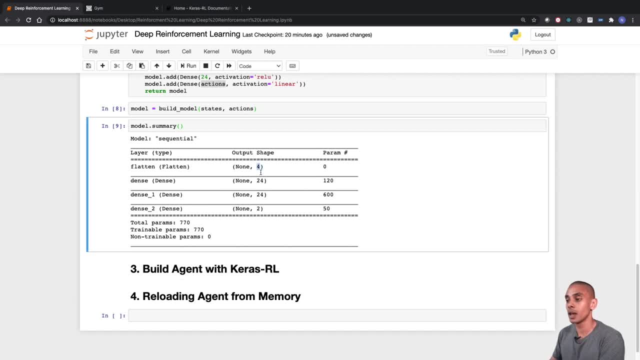 so you can see here that we're passing through our four different states. we've got 24 dense nodes- 24 dense nodes, so these are going to be our fully connected layers within our neural network. and then, last but not least, we're going to be passing out our two different actions that we 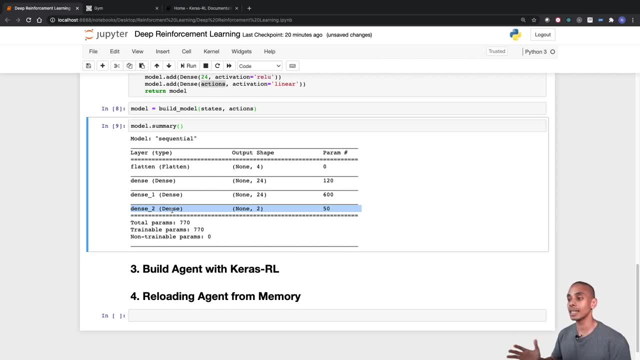 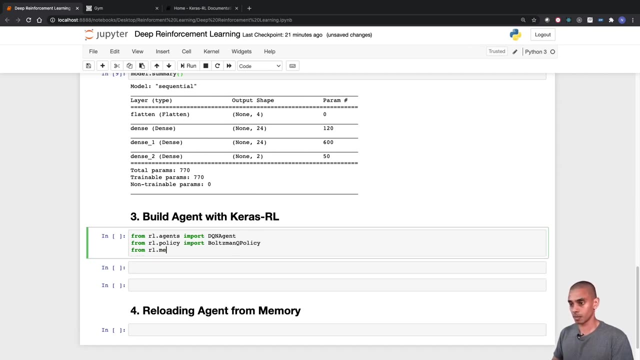 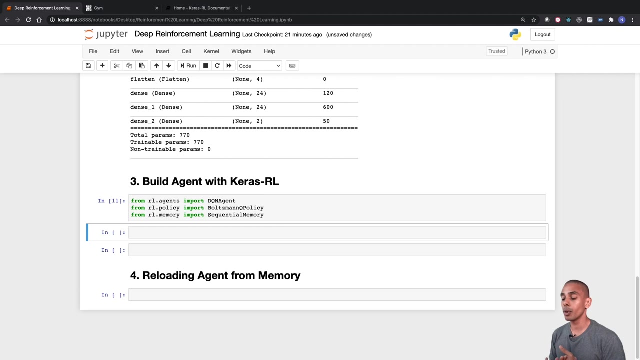 want to take within our environment. now what we can go and do is take this deep learning model and actually train it using Keras RL. so, first up, we need to import our Keras RL dependencies. so let's go on ahead and do that. so those are our dependencies imported. so we've imported three key things here. so we've imported. 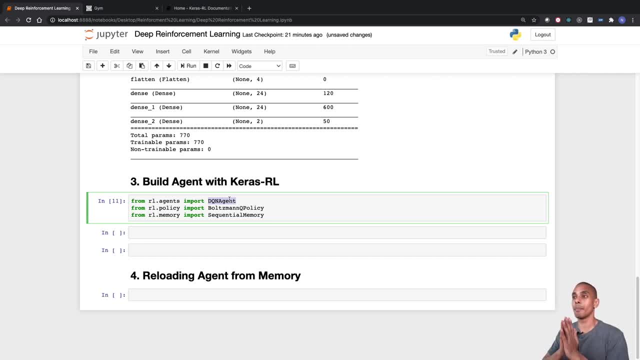 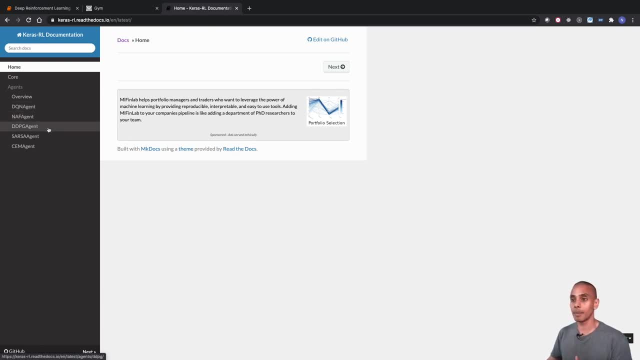 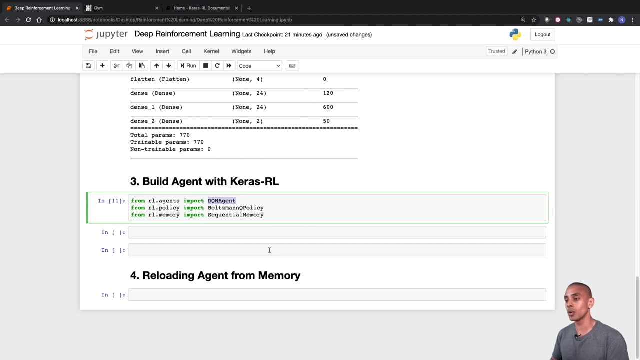 our DeepQ network agent. so basically there's a bunch of different agents within the Keras RL environment. so you can see we've got a DQN agent, a NAFA agent, a DDPG, Sasa, SEM. so all of these are different agents that you can use to train your reinforcement learning model. we're going to 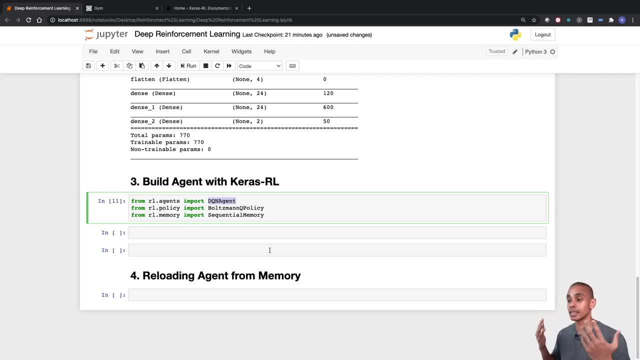 be using Keras RL to train your reinforcement learning model, and we're going to be using DQN for this particular video, but try testing out some of the others and see how you go. now what we also have is a specific policy. so within reinforcement learning, you've got different. 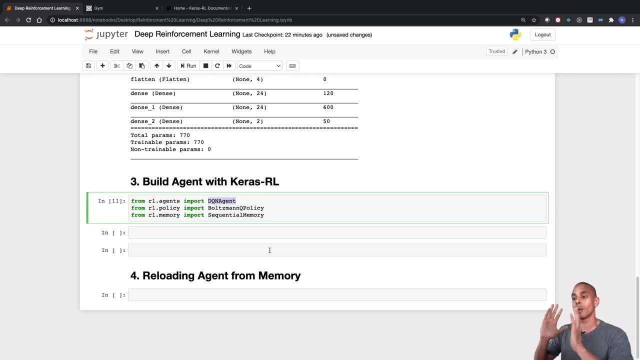 styles. so you've got value-based reinforcement learning and you've also got policy-based reinforcement learning. so in this case, we're going to be using policy-based reinforcement learning, and the specific policy that we're going to be using is the Boltzmann Q policy, which you can see here. now, the last thing that we've gone and imported is sequential memory. so 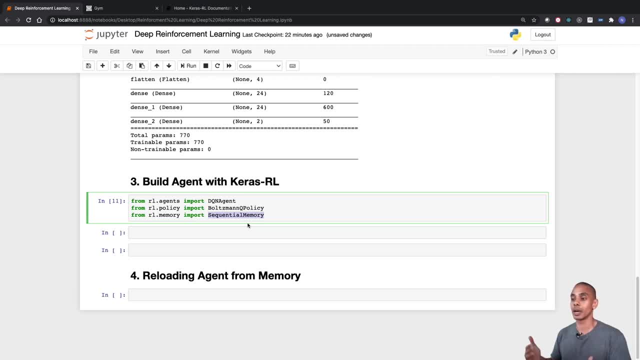 for our DQN agent, we're going to need to maintain some memory. so we're going to need to maintain some memory. so for our DQN agent, we're going to need to maintain some memory, and the sequential memory class is what allows us to do that. so now what? 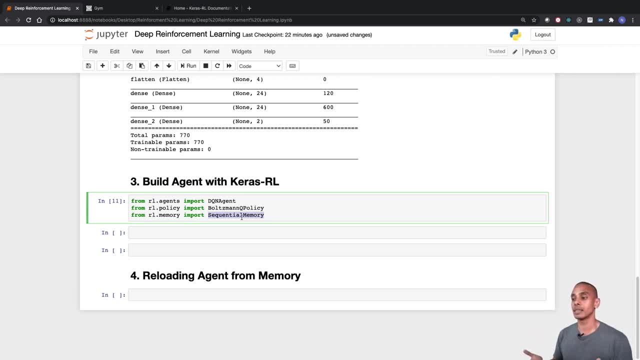 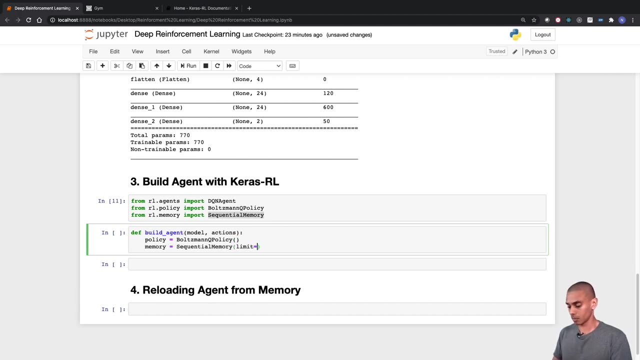 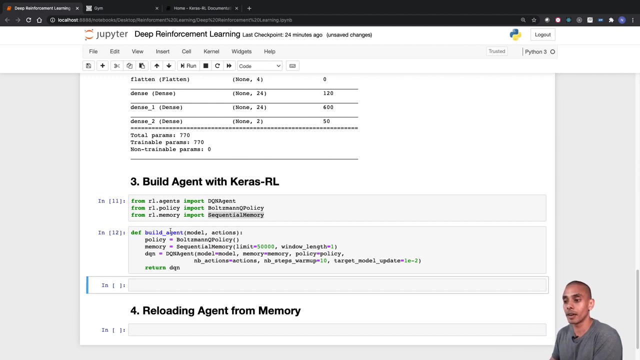 we can go and do is set up our agent, and again, we're going to wrap this inside of a function so we can reproduce it when we want to reload it from memory. so let's go on ahead and build that function. so that's our function defined. now, what we've basically done is we've named our function, build. 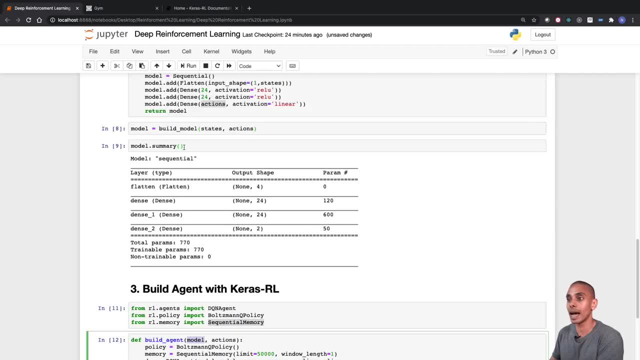 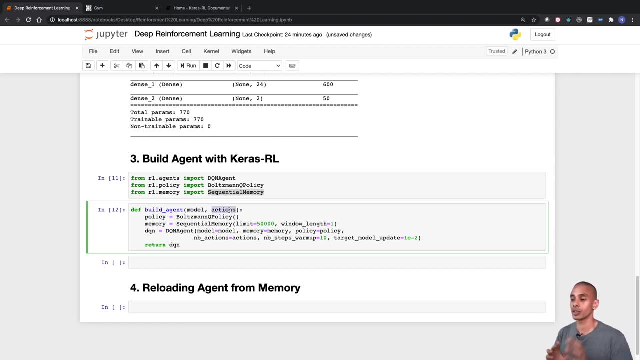 agent and to that we pass through our model. so this is our deep learning model that we specified up here, and we're also passing through the different actions that we can take. so those were the two different actions, left or right, that we had available within our environment. 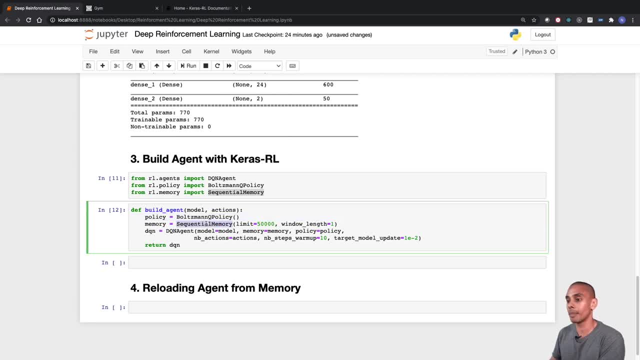 then we set up our policy and we're going to go ahead and build that function and we're going to. we set up our memory and we set up our DQN agent and to that DQN agent we actually pass through our deep learning model and memory, our policy as well as a number of other keyword arguments. so then, 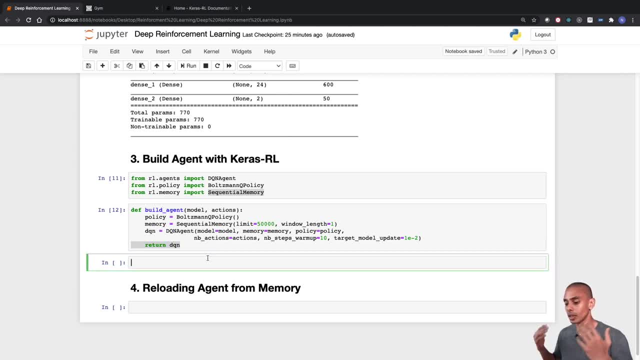 what we do is we return that DQN agent. so let's go on ahead and actually use this DQN agent to actually now go and train our reinforcement learning model. so first up, we want to start out by instantiating our DQN model. then we're going to compile it and then we're going to go. 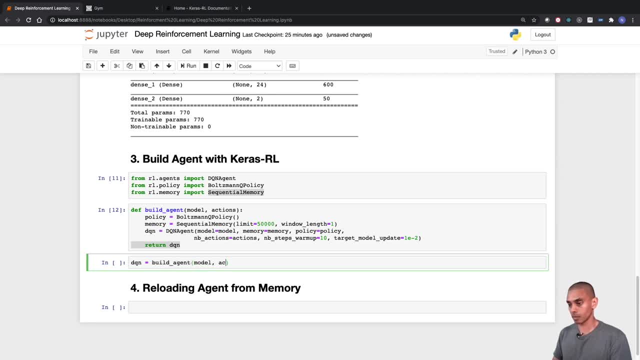 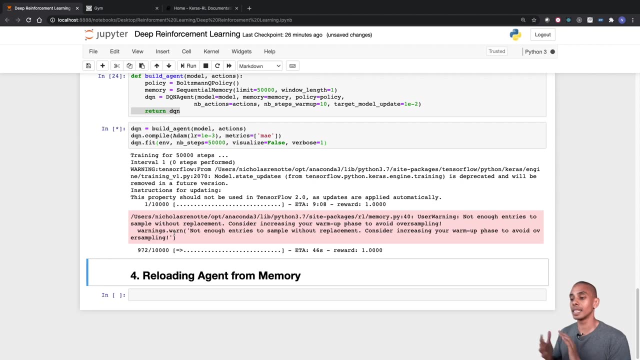 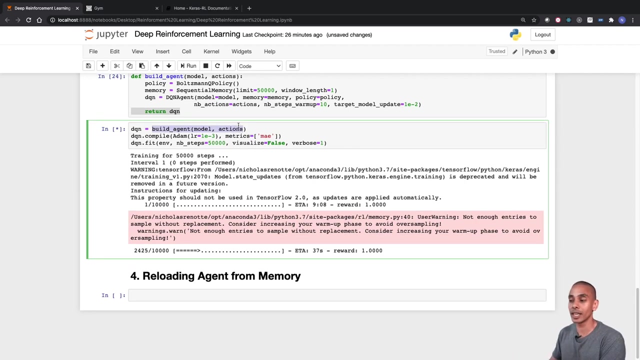 ahead and fit it all right. and there you go, so you can see that our DQN model is now starting to train. so what we actually did is we instantiated our, or we used our build agent function to set up a new DQN model, and that was that up here, and we pass through our model as well as our actions. 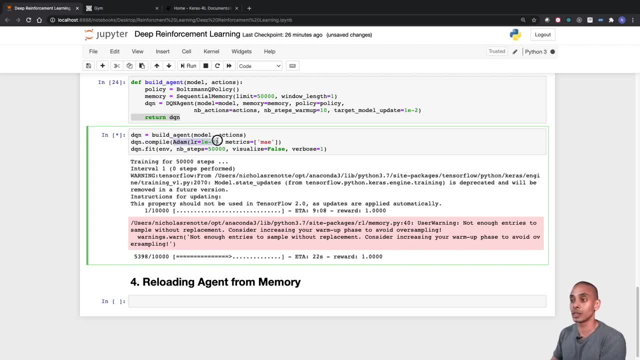 and we're going to go ahead and set up our DQN model- and that was that up here- and we pass through our model as well as our actions. we then compiled it and we pass through our optimizer. so this was that atom optimizer that we imported right at the start, and we also pass through the metrics that we 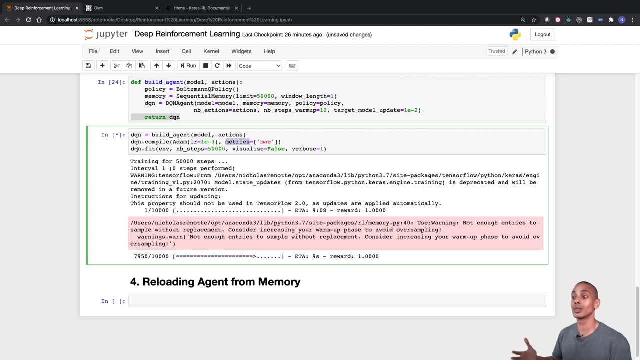 want to track, so in this case it's mean absolute error. then we use the fit function to kick off the training and to that we pass through our entire environment the number of steps we want to take, whether or not we want to visualize it. so we'll take a look at that in a second, and we also 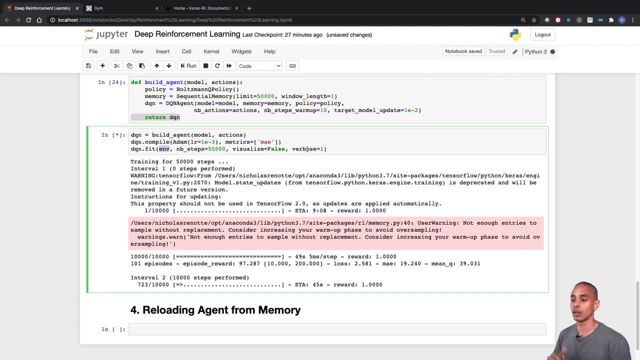 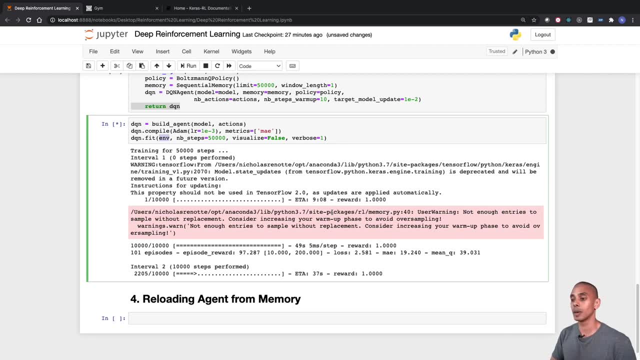 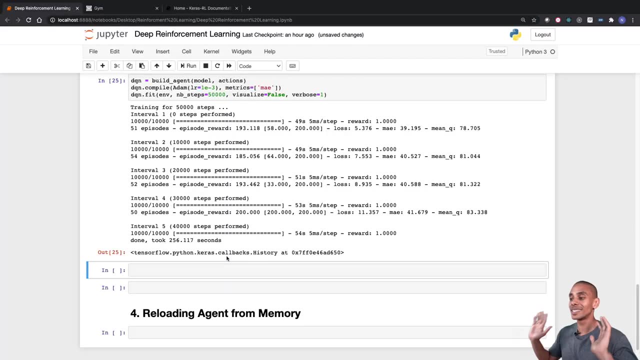 specified verbose as one. so we don't want full logging, we want a little bit of logging. now what we can do is just let that go ahead and train, so take a couple of minutes and then we should have a fully built reinforcement learning model five minutes later. sweet, so that's our reinforcement learning model, now done, dusted and trained. so all. 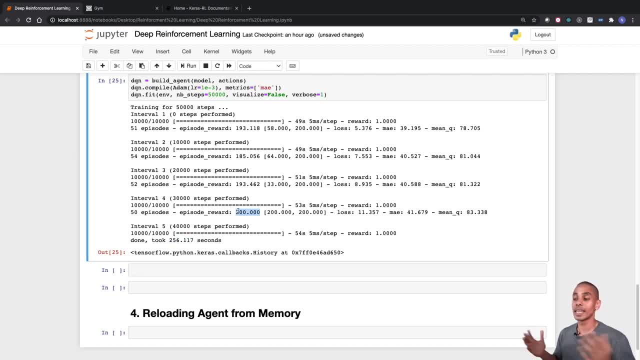 up. it took about 256 seconds to go and train and you can see in our fourth interval that we're accumulating a reward of about 200. now what we can go and do is actually print out and see what our total scores were. so remember when we started out up here- so just taking random steps we were- 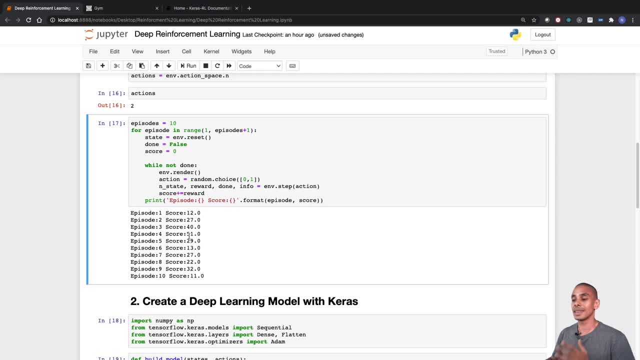 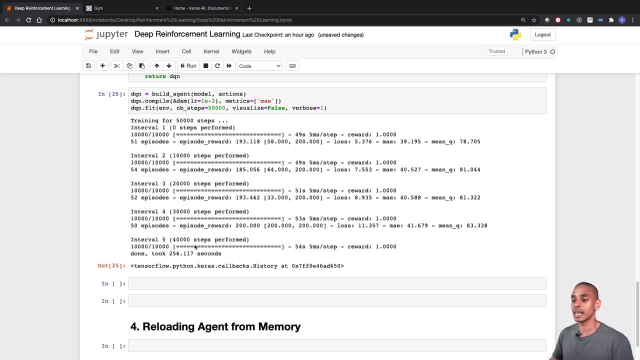 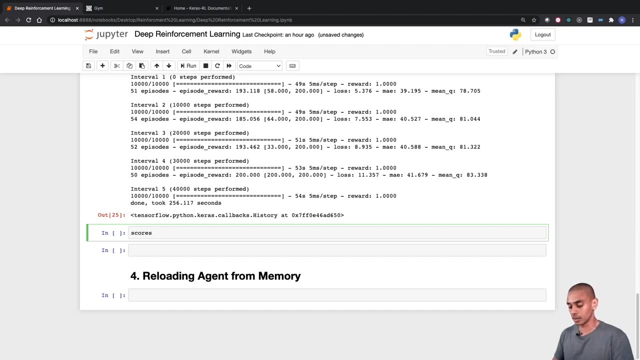 getting about a maximum score of about 200, and then we're going to go ahead and train and we're going to go ahead and test this out and see what this actually looks like or how it's actually performing. so we can do that using the dqntest method. so let's try that out. 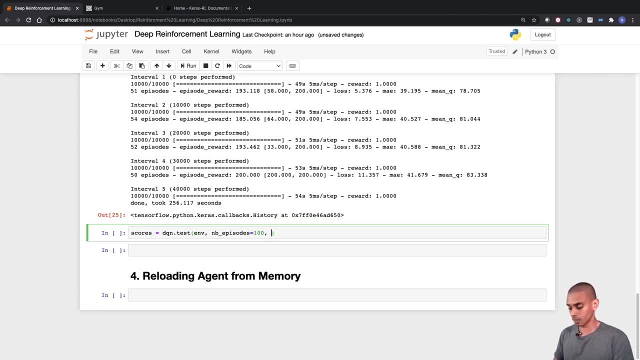 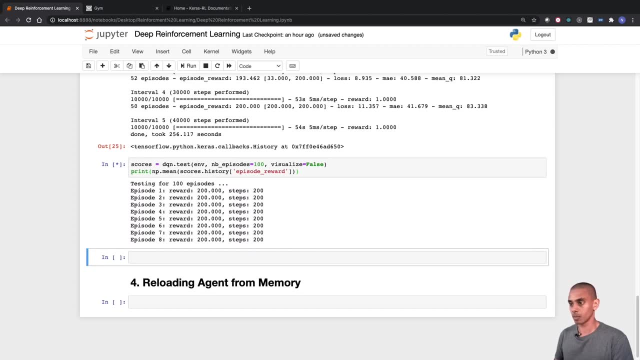 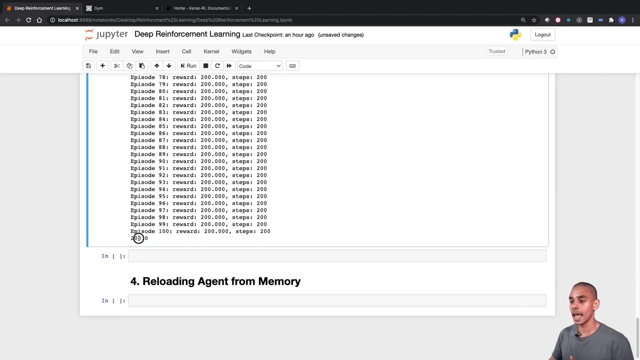 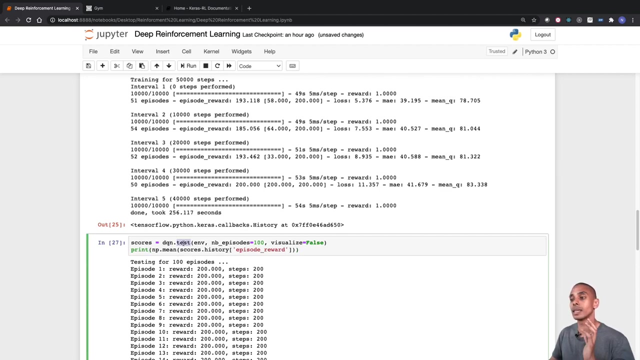 all right, so that's looking better already. so you can see that the total score for the game is about. we're getting a score of about 200 and our mean is 200. so what we did there in order to test that out is: we accessed our dqn model and we use the test method to that we pass through our actual. 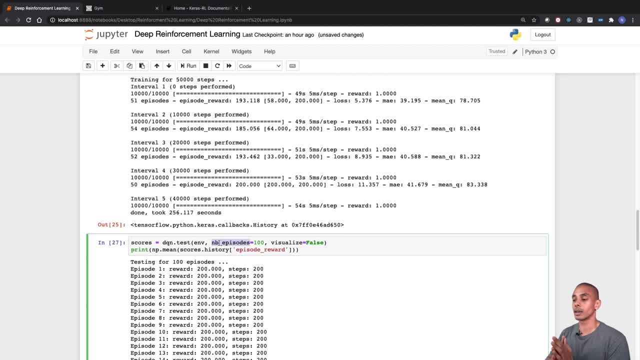 environment, the number of games that we want to run, so in this case they're called episodes. so we ran 100 games and, whether or not we want to visualize it then what we did is we outputted our mean result. now, if we wanted to actually visualize what the difference is, we can do that. 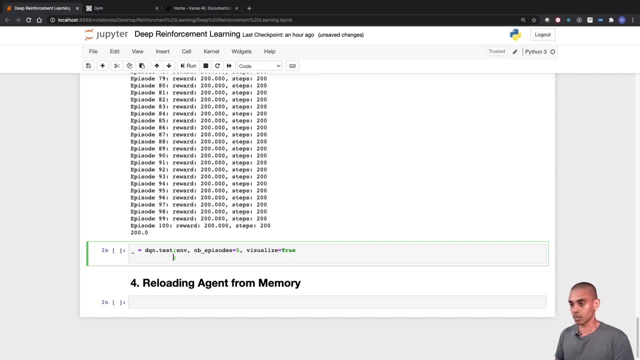 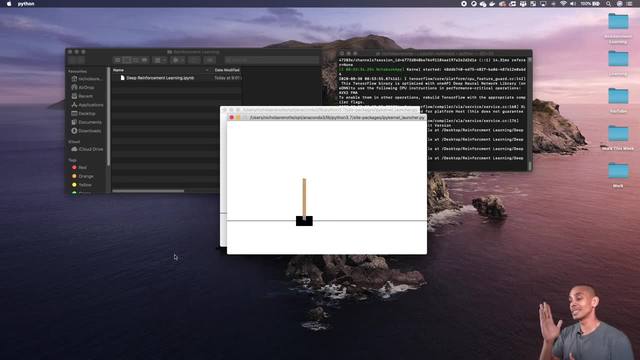 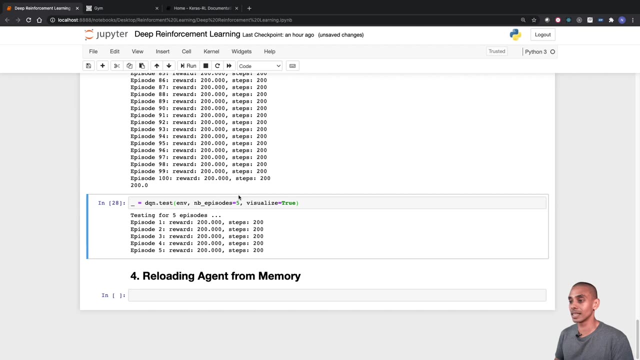 by just clicking on the model and we can see that our model is performing way better. so you can see it's actually able to balance the poll a whole lot better than what it was before, when it was just randomly sort of flailing about. we can test that out again. so this time, rather than doing five. 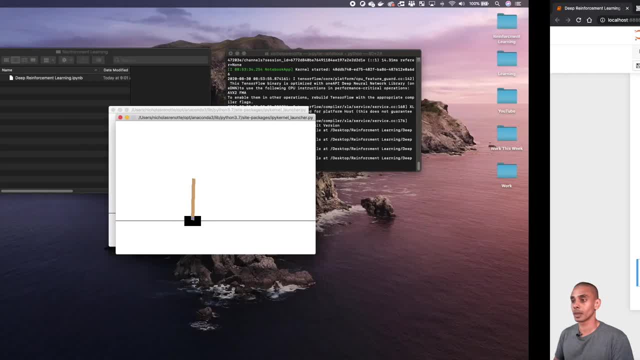 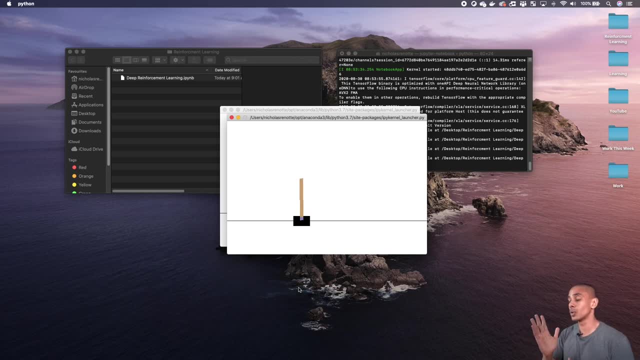 episodes, say we wanted to um 15, for example. so you can see that our model- again it's performing way better than what it was initially, so it's actually able to run a lot of the game and we can see that our model is actually able to balance the poll a whole. 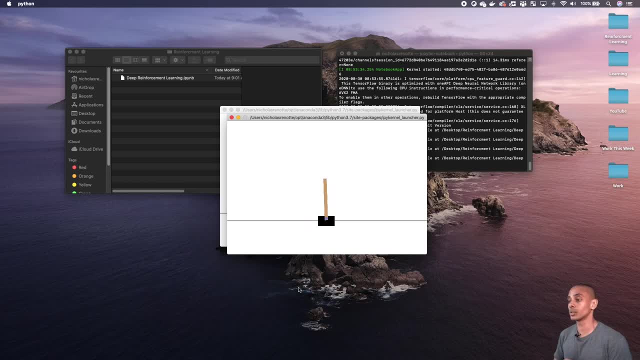 lot better than what it was initially. so we can see that our model again. it's performing way better than what it was initially. reiterate itself and re-sort of balance to make sure that that poll stays straight brings a tear to my eye. so good, sweet. so that's all done. now what happens if we actually wanted to go and save this model away? 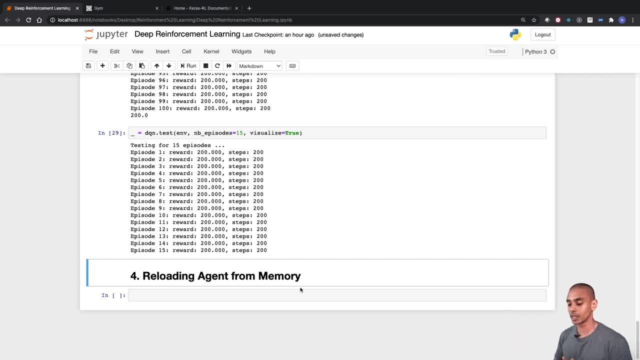 and use it later on. say, for example, we wanted to go and deploy it into production. well, what we can actually do is we can actually save the weights from our dqn model and we can actually- uh, we can- run a few files into our dqn model so we can use that, the save parts from our dqn model. 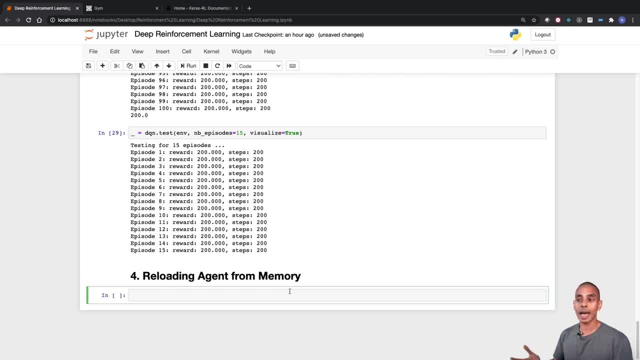 and then reload them later on it to try to test them out. so we can do that using the save weights: елься specie черезseokmodel- fraic bestpwickings part from our dqn model. so we can do that using the savethat, The Save weights method from our dqn model. so 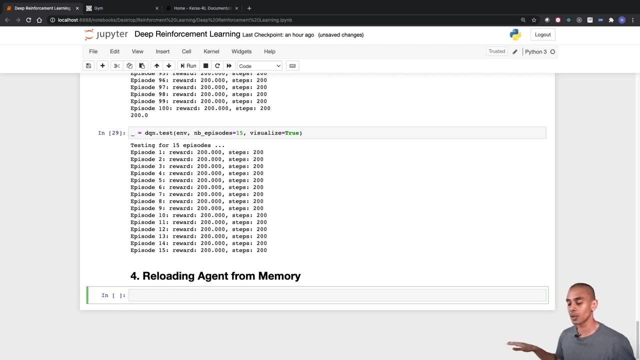 let's go on ahead and save our weights. so let's go ahead and save our weights. then what we'll do is we'll blast away all of the stuff that we just created. and we'll blast away all of the stuff that we just created, and we'll 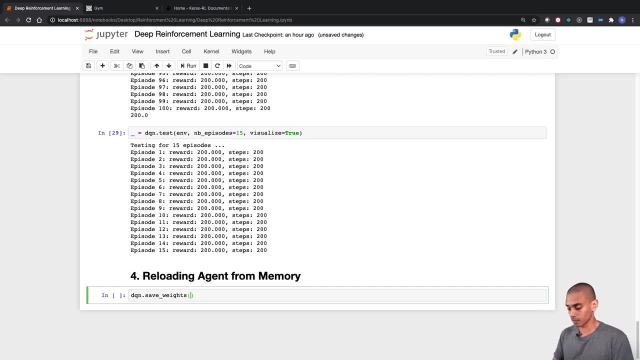 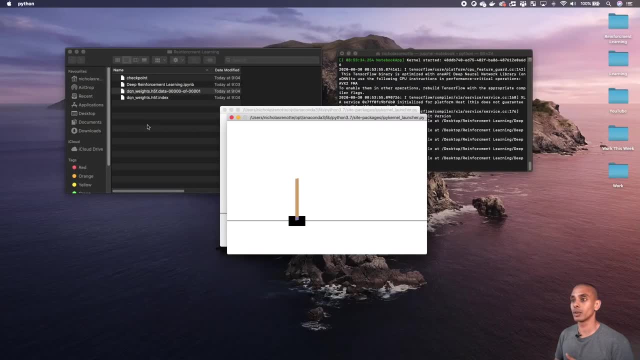 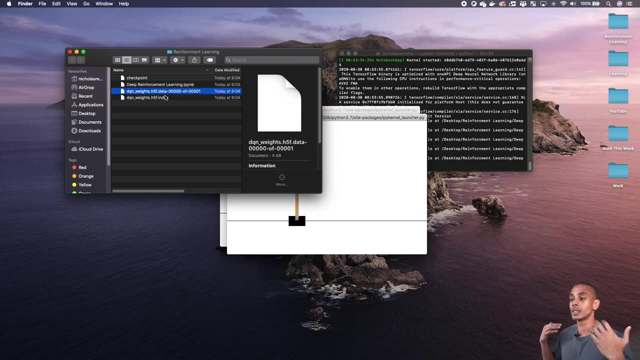 rebuild it by reloading our weights. so we've now gone and saved our weights. so if we actually take a look in our so if we actually take a look in our folder, you can see that we've gone and generated two different h5f files. so these basically allow us to save our reinforcement. 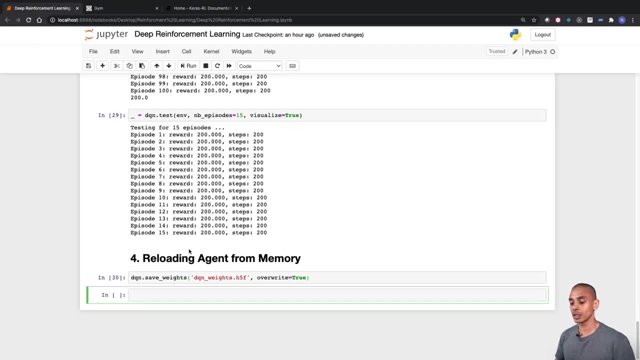 learning model weights. now, if we wanted to go and rebuild our agent first up, let's start by deleting our model, deleting our environment and deleting our dqn agent, and then what we can do is rebuild it using all the functions that we had and reload those weights to test it out. so if we 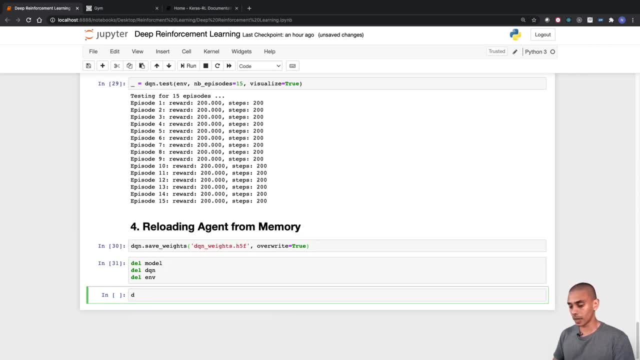 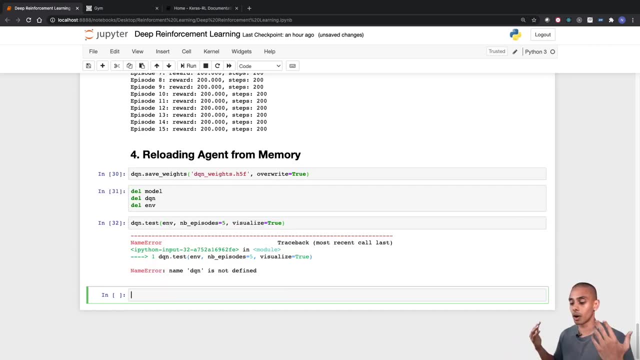 go and do that so you can see if we go and try to use our dqntest method. there's nothing there, because we've then gone and deleted it, but what we can do is we can go and rebuild that environment and test it out. so let's go and do that. 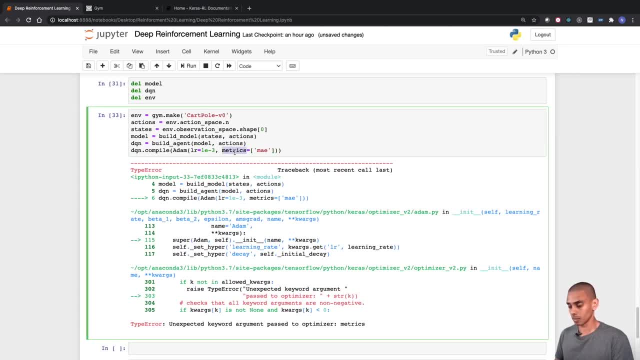 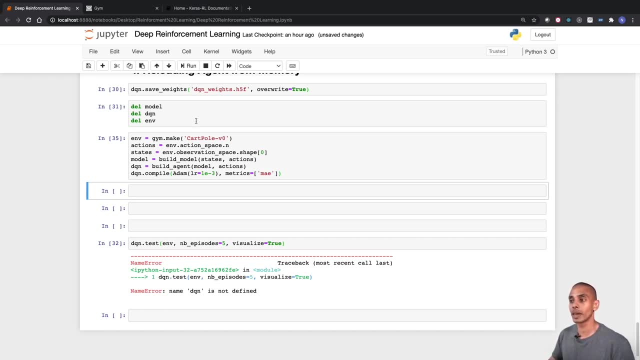 perfect. so we've now gone and reinstantiated all of our models. so we first up, we built our environment, we extracted our actions and our states, just like we did before. then we used our build model and our build agent functions to go and rebuild our deep learning model and 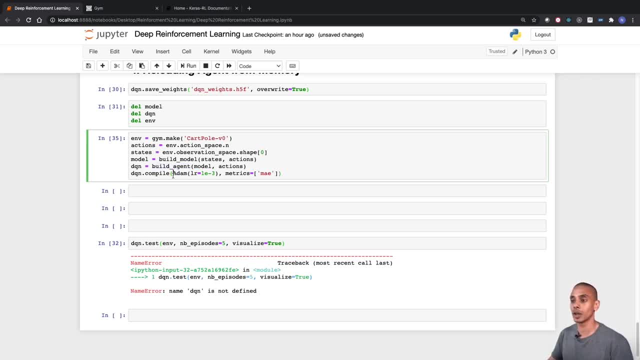 reinstantiate our dqn agent and then, last but not least, we compiled it. now what we can do is actually reload our weights into our model and then we can go and reinstantiate our dqn agent model and then test it out again. so in order to do that, we can use the dqnload weights method. 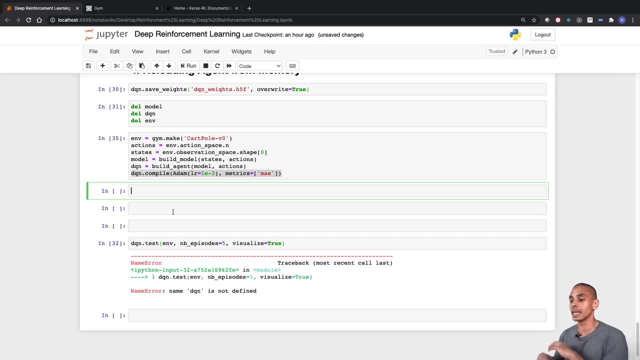 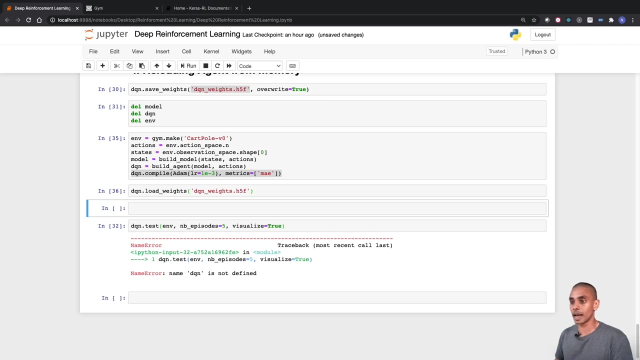 so before up here, we use save weights. now we can load our weights in order to retest this out, and the file that we're going to pass to our load weights method is the one that we exported out here, so we can copy that in and paste that here, and now we've gone and reloaded our weights. we. 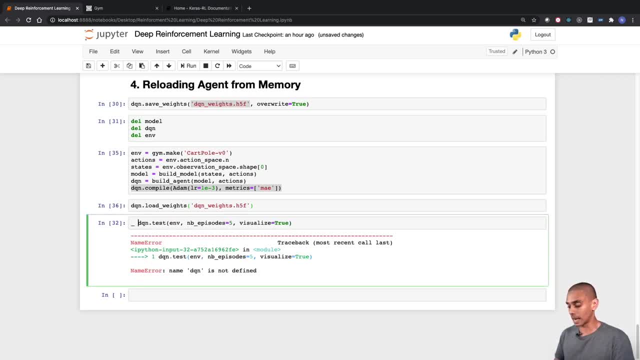 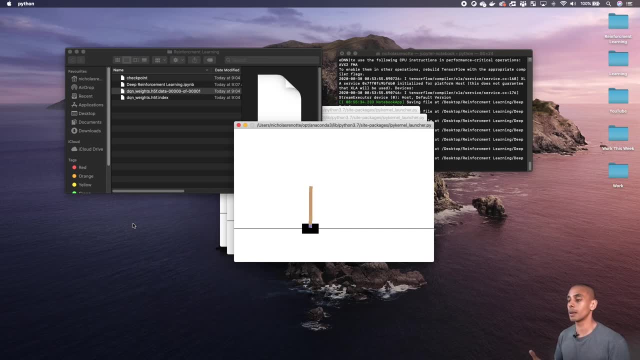 can actually go and test out our environment again. so ideally, what we should get is similar results. so again, you can see it's performing well. it's performing just as well as what it did before. we deleted our weights, and now we went and reloaded them, and that about wraps up this. 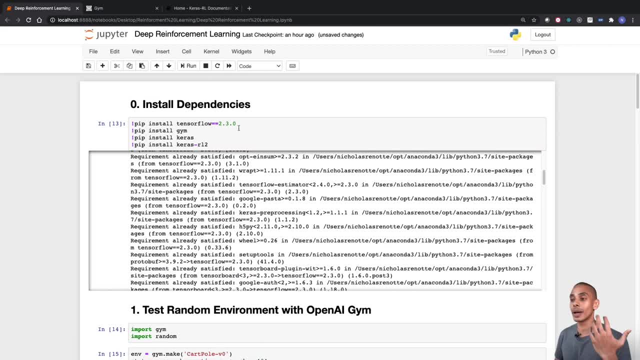 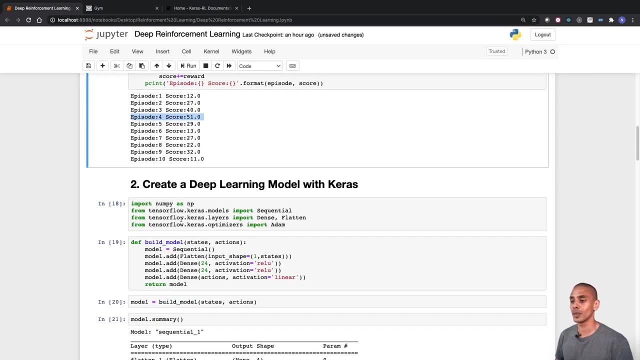 video. so we covered a bunch of stuff. so, specifically, we went and installed our dependencies, we then created a random environment using openai gym and we got about a maximum score of about 51. we then built a deep learning model using keras and then used keras rl to train that. 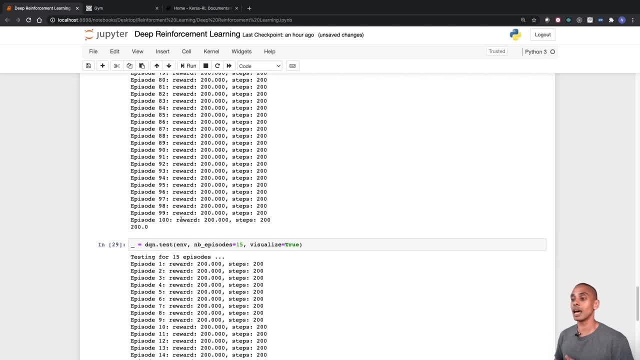 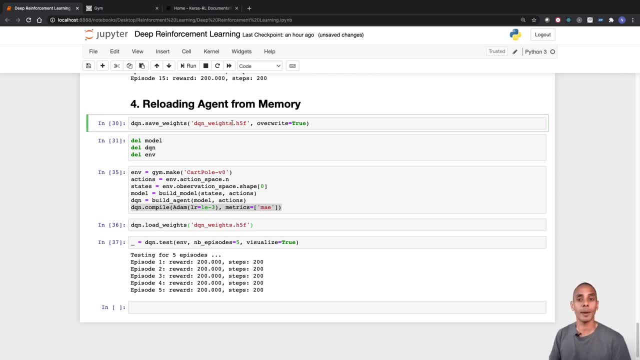 using policy-based reinforcement, learning. and then, last but not least, we went and reloaded that agent from memory, so that allows you to work with this inside of a production environment if you want to go and deploy it. and that about wraps it up. thanks so much for tuning. 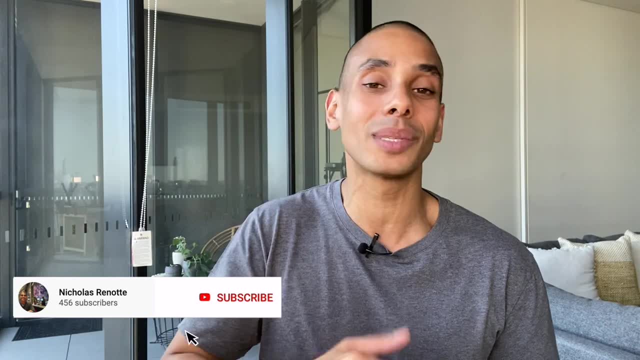 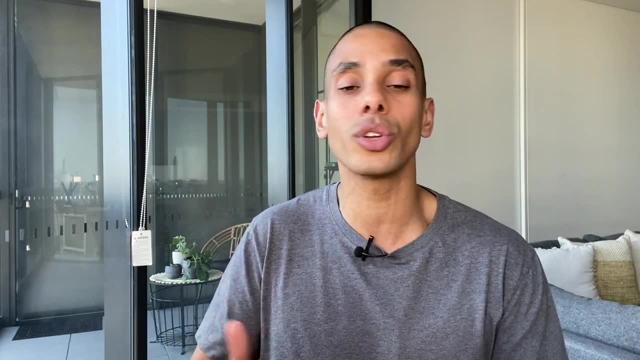 in guys. hopefully you found this video useful. if you did, be sure to give it a thumbs up, hit, subscribe and tick that bell so you get notified of when i release future videos. if you do have any questions or need any help, be sure to drop a mention in the comments below and i'll get right. 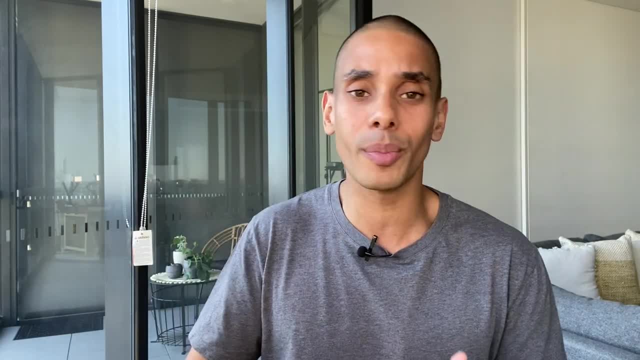 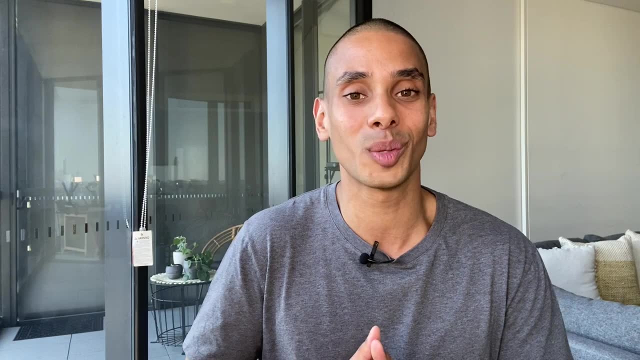 back to you, and all the course materials, including the github repository, as well as links to documentation, are available in the description below, and i'll see you in the next video. bye, bye, so you can get a kick start and get up and running with your reinforcement learning model. 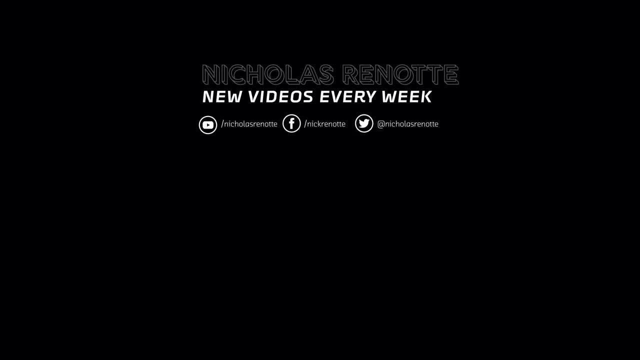 thanks again for tuning in peace.